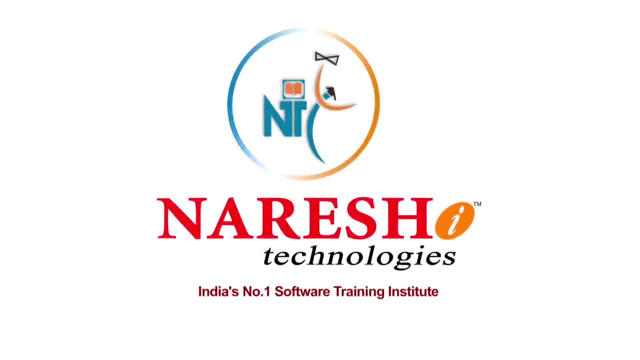 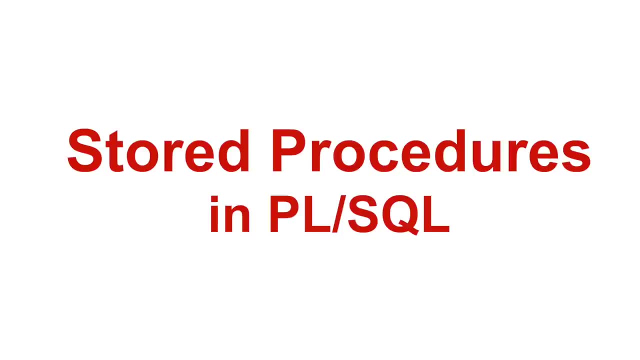 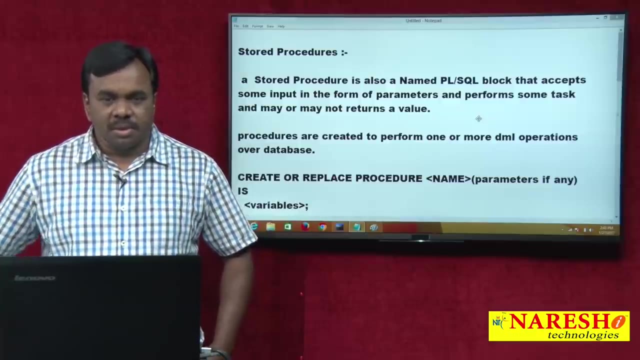 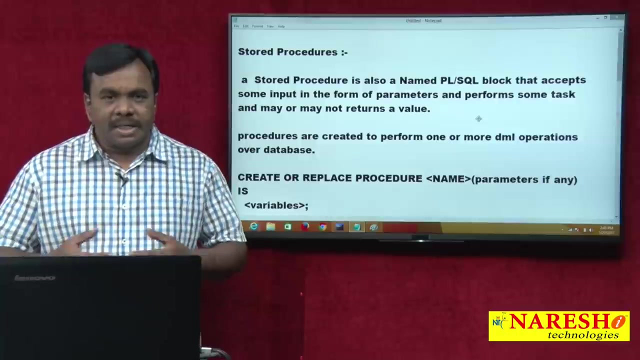 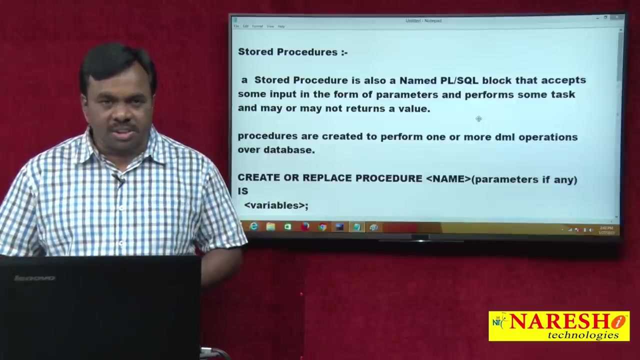 This is Vijay Kumar from Naresh Technologies and today's session, and I am going to explain about procedures- stored procedures, One of the most important topic in PLSQL. In previous video so I explained about functions and today's video I am going to explain about. 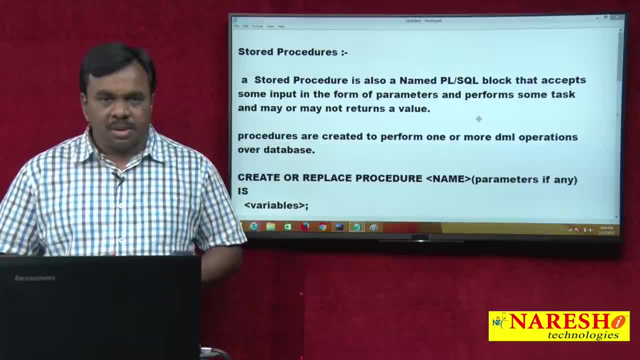 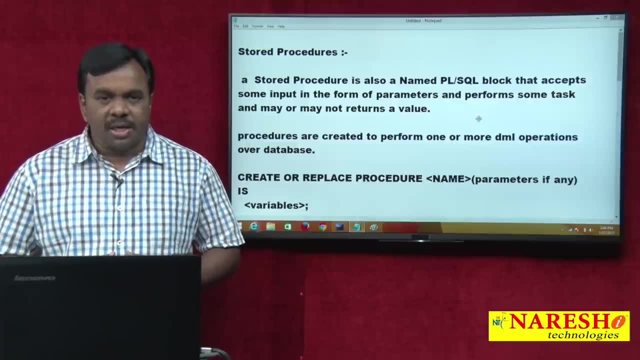 procedures, stored procedures. So what is stored procedures and what for stored procedures are created. A stored procedure is also a named PLSQL block. It accepts some input with the help of parameters and perform some task, and may or may not returns a value. 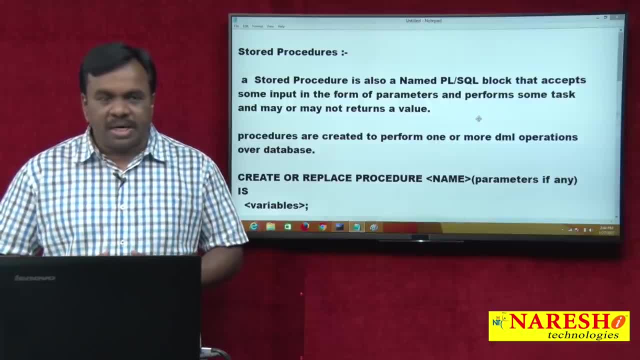 A stored procedure is also a named PLSQL block that accepts some parameters in the form of that, that accepts some input in the form of parameters and may or may not returns a value. So what for stored procedures are created, And stored procedures are mainly. 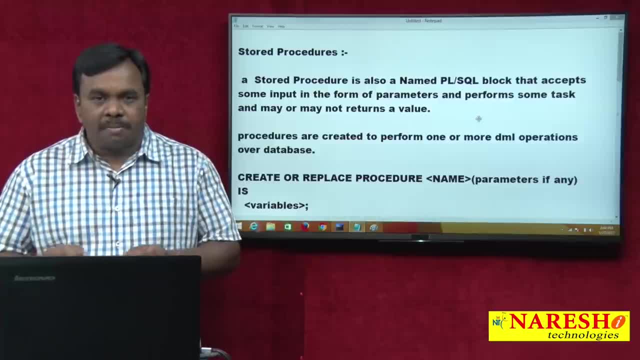 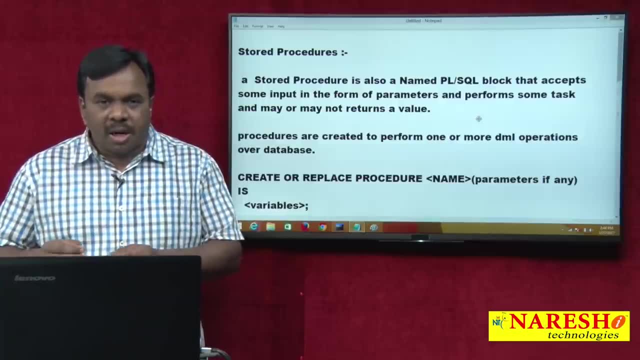 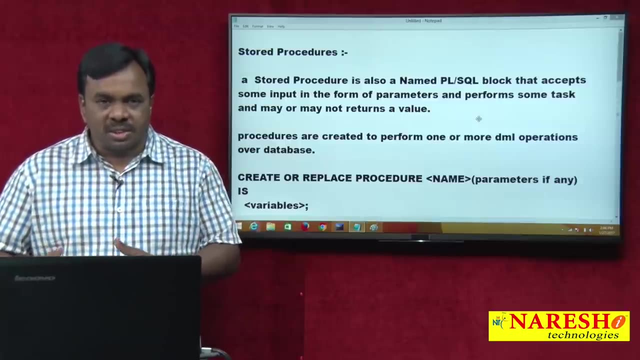 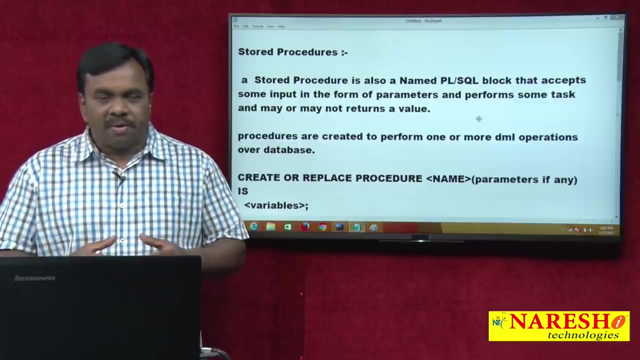 created to perform one or more DML operations over database. So to perform one or more operations over DML operations over database. We create stored procedures like, for example, I want to insert, I want to update, I want to delete, So I want to perform this- insert and update. or I want to perform update and 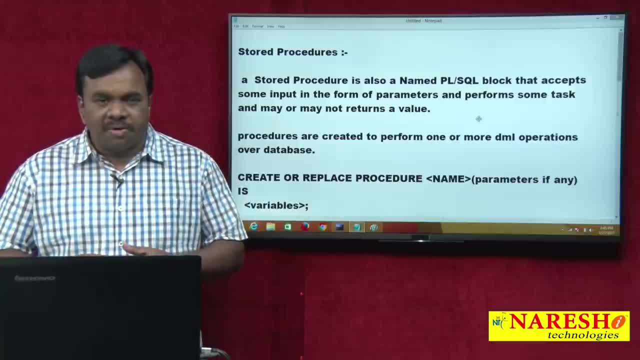 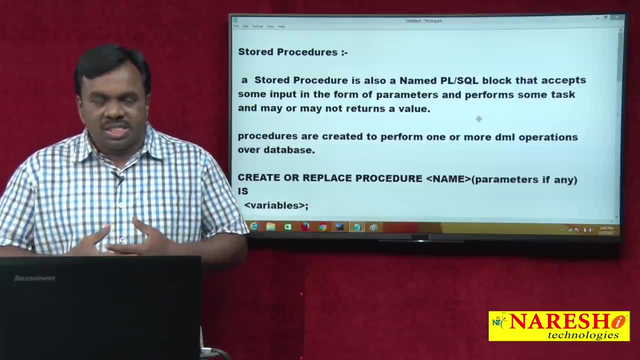 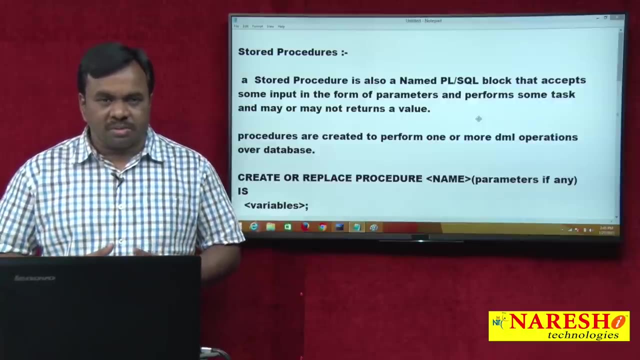 delete or I want to perform delete and insert, So to perform one or more DML operations over database. we create stored procedures. So in this session we will see how to create a stored procedure and how to execute the stored procedure And what is the syntax for creating the stored procedure. and the syntax is create. 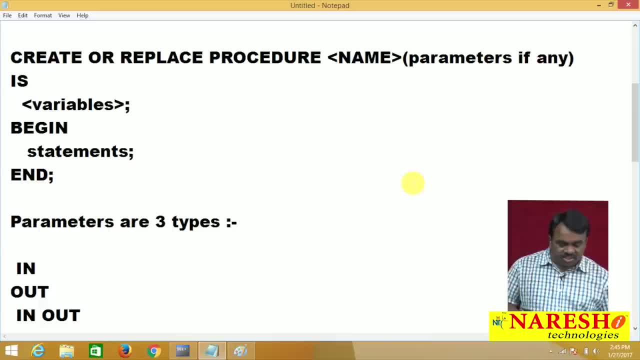 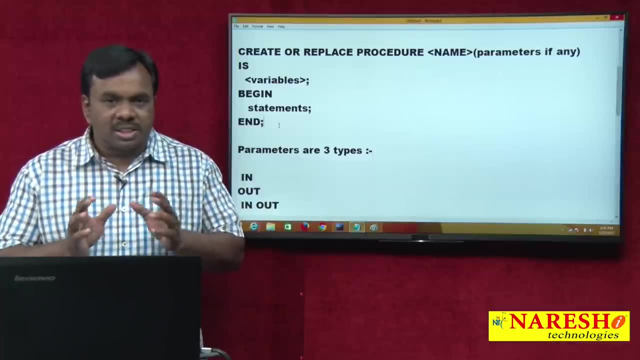 or replace procedure procedure name parameters, if any. Create or replace procedure procedure name parameters, if any is variables begins statement send. that is all The simple. So just creating stored procedure is as simple as a normal PLSQL program. So create or replace. 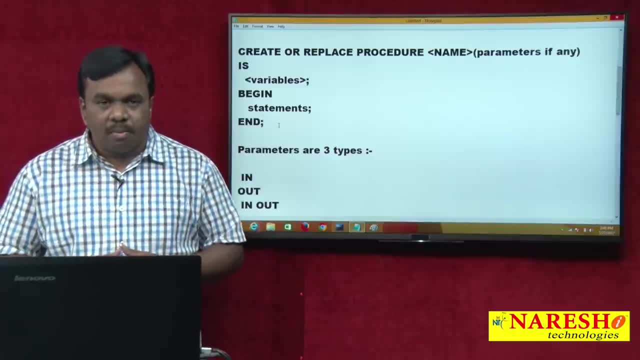 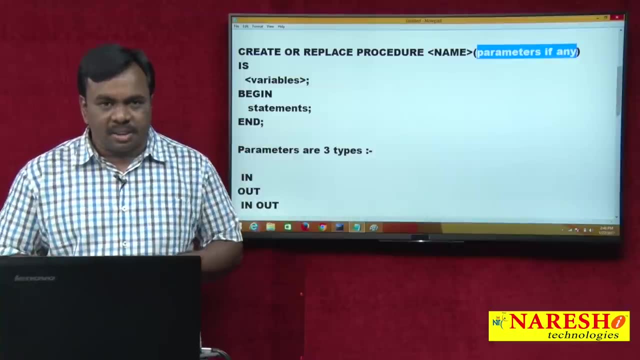 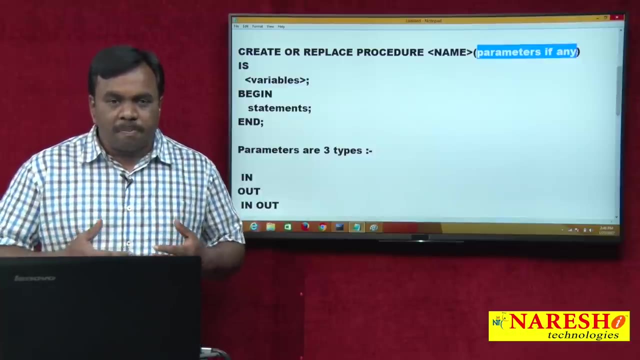 procedure, procedure name, parameters, if any, And the most important part in creating stored procedure is parameters. The most important part is parameters. So what for? we use parameters And parameters are mainly used to pass values. We declare the parameters and we pass values. 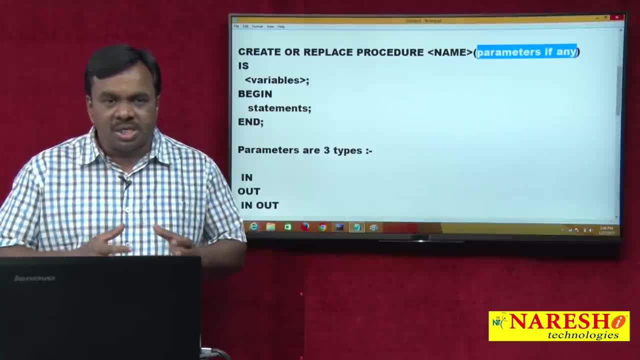 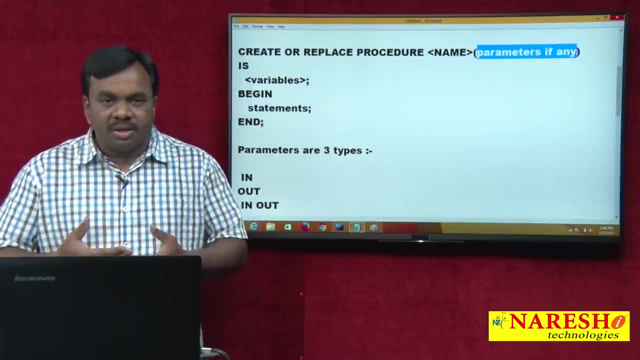 to the parameters. The purpose of using parameters is to pass values. So in normal PL SQL program, like anonymous block, how you input the values by using ampersand, substitution variables using ampersand. But when it comes to procedures, how you input the values using parameters. 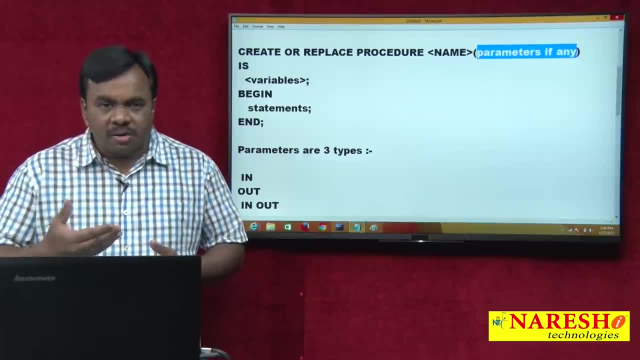 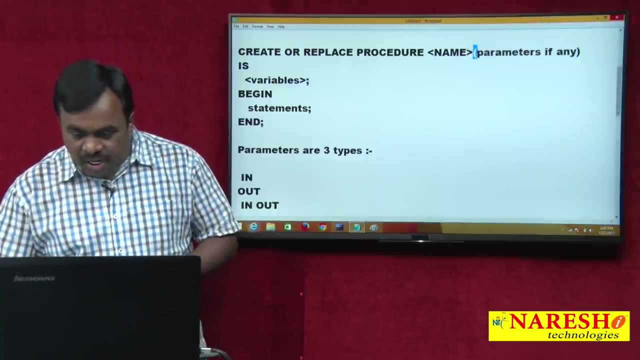 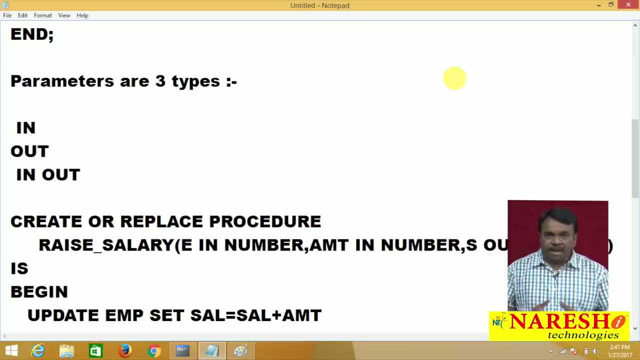 If you want to pass some value to the procedure, you can pass values to the procedures in the form of parameters. So we declare the parameters and we can pass values to the parameters. So these parameters are mainly three types: One is in parameter, another one out parameter and another one. 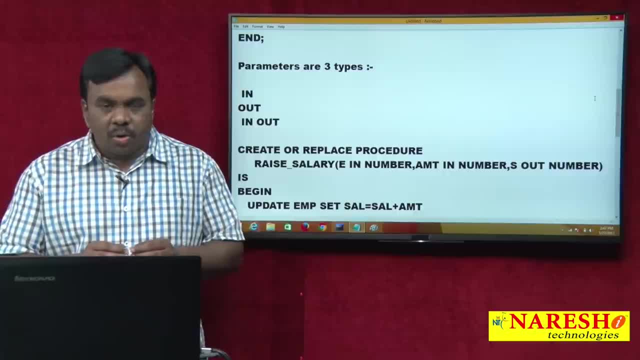 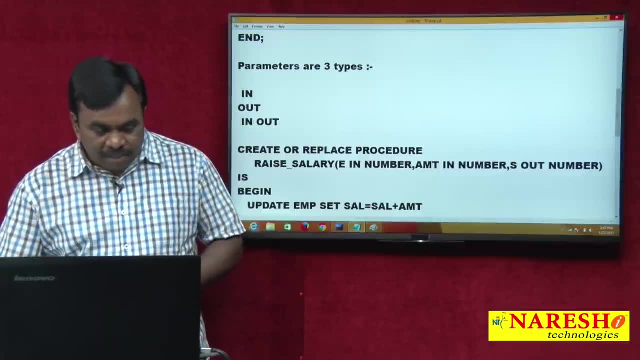 in out parameters. So and if you do not declare any type, for example, if you do not mention in out in out, by default the parameter is in parameter, So in is what Default. So if you do not declare the parameter type? 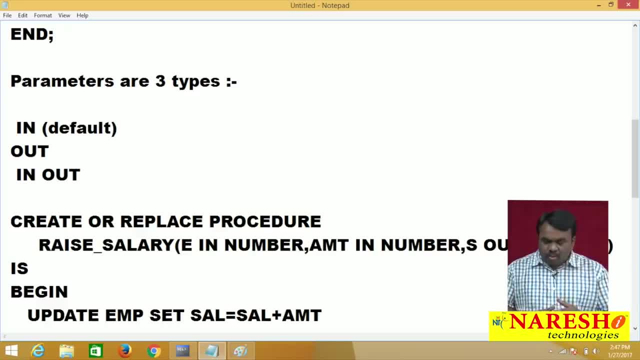 By default, the parameter is in parameter. So then, what is this in, what is this out and what is this in out? So in parameter always receives value. out parameter always sends value and in out parameter receives as well as sends. So in parameter always. 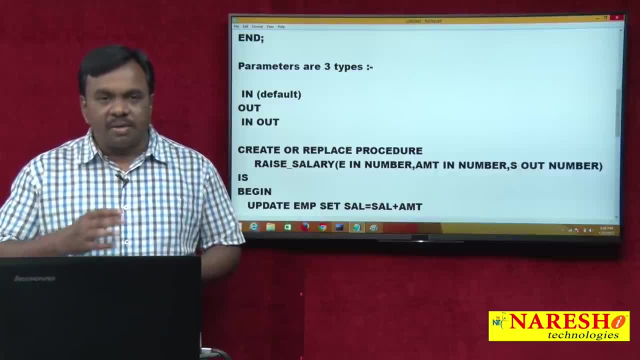 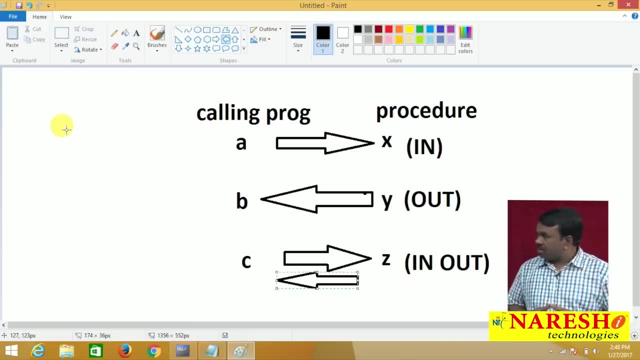 receives value and out parameter always sends value and in out parameter receives as well as sends. So let us see this diagram. Then assume I created a procedure and the. in that procedure I declared three parameters. one parameter is x, one parameter is y, one parameter is z, and what is x is x is in parameter. 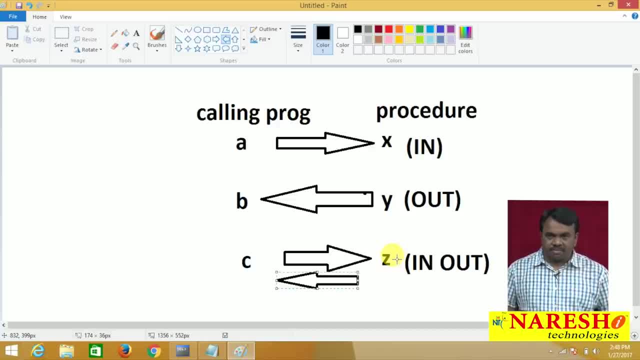 and y is out parameter and z is in parameter next. So I created a procedure with three parameters and after that the procedure is executed from some program. We create the procedures, because this procedures and functions are called subprograms. We create the subprograms. 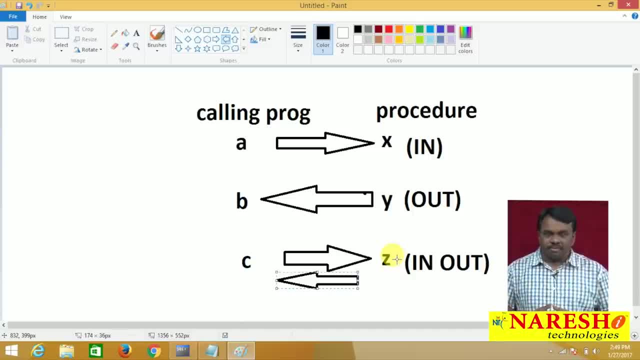 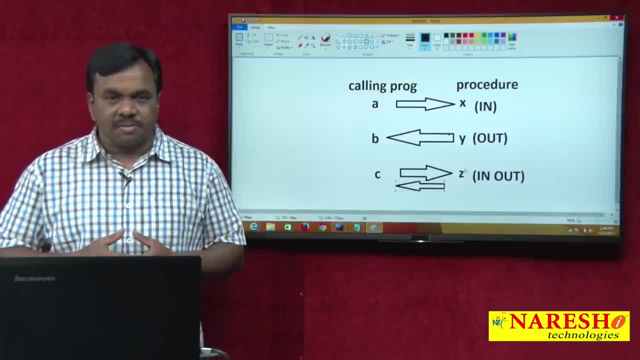 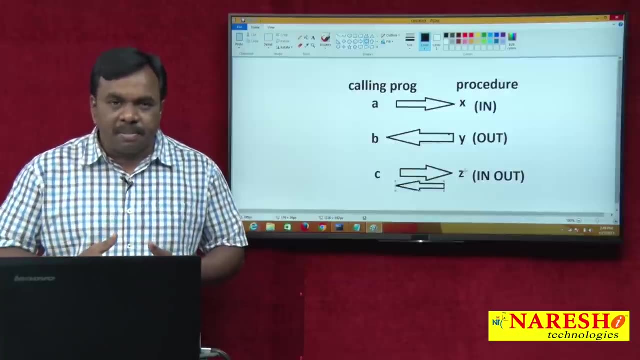 and the subprograms are executed from some other program, So that program is called calling program. What is calling program is The program that is calling the procedure, So that can be another PLSQL program, or that can be Java program, or that can be a dotnet. 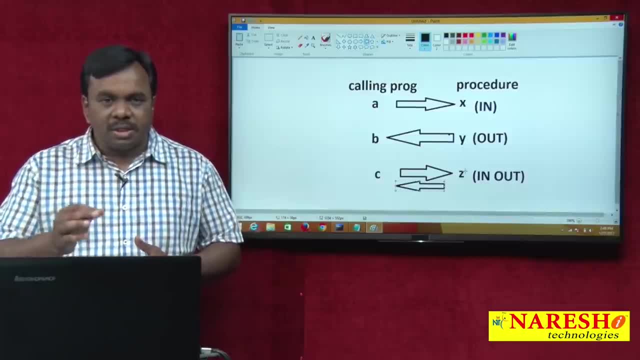 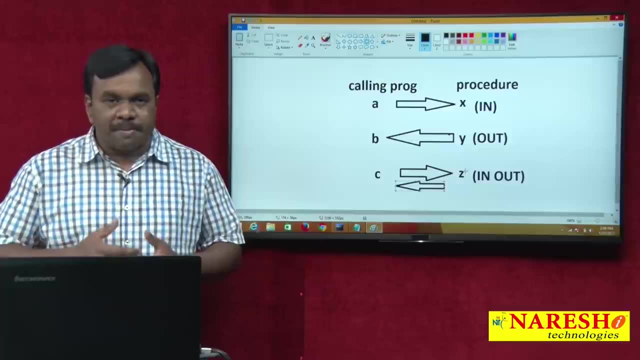 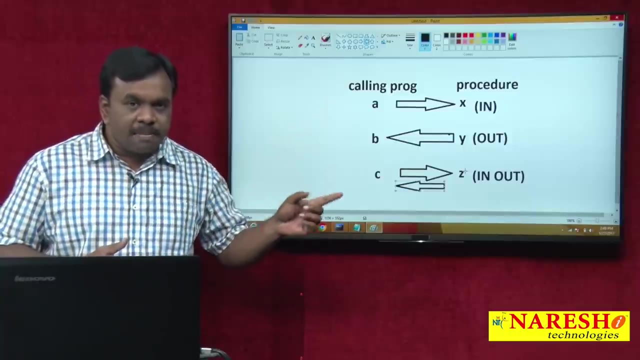 program. So the program that is calling the procedure is called calling program. So the program is calling the procedure, and the procedure should be invoked with three parameters. So the procedure is invoked with three parameters: a, b, c. The procedure is created with three parameters- x, y, z- and the procedure is called 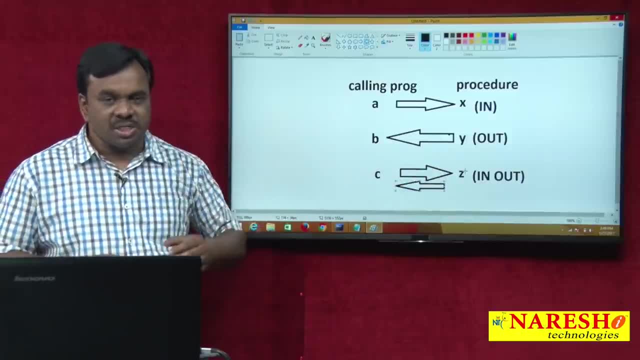 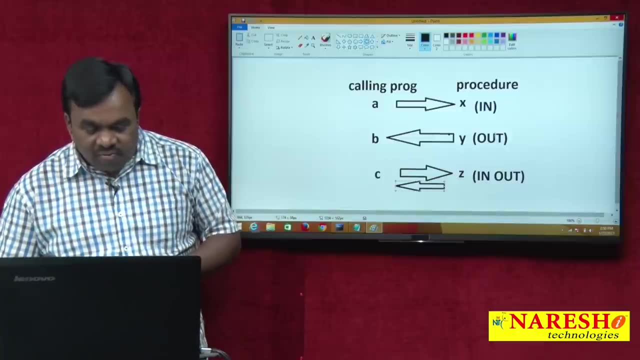 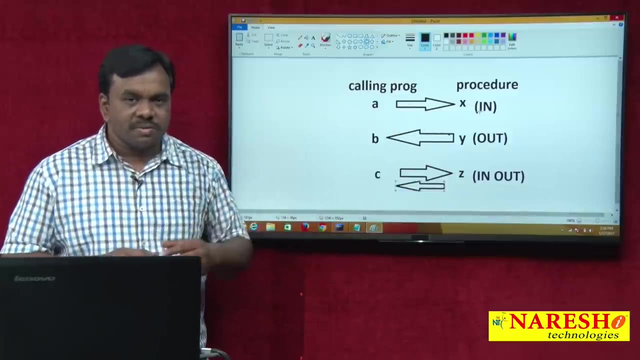 with three parameters, and the three parameters are a, b, c. So then when this procedure is executed, then the value of a is passed to x Because x is in parameter. the value of a is passed to x because in parameter always. 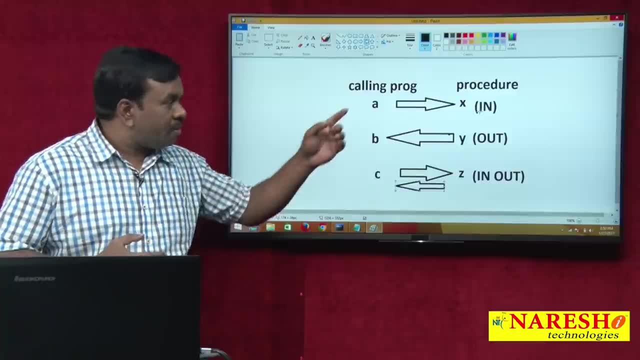 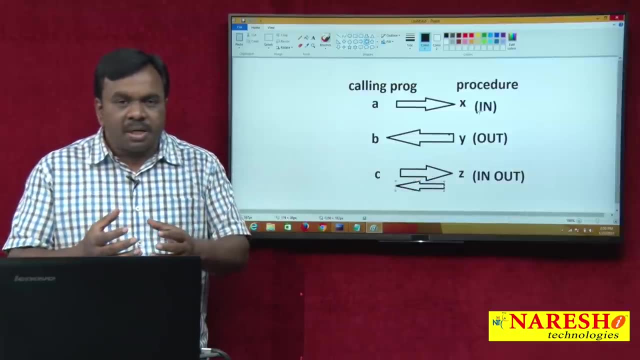 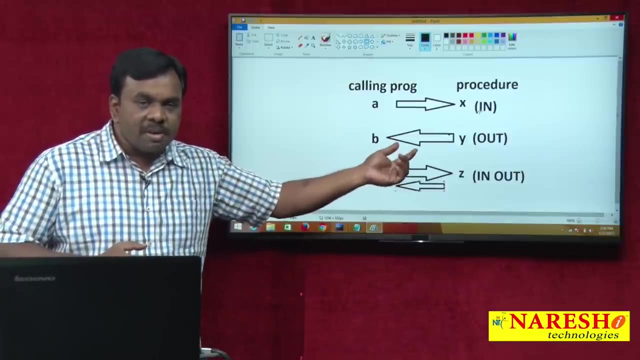 receives value from calling program. So from the calling program the value of a is passed to x. Next y is out parameter. Out parameter always sends a value, So y is sending the value. So the parameter b receives the value that is coming from procedure Out parameter. 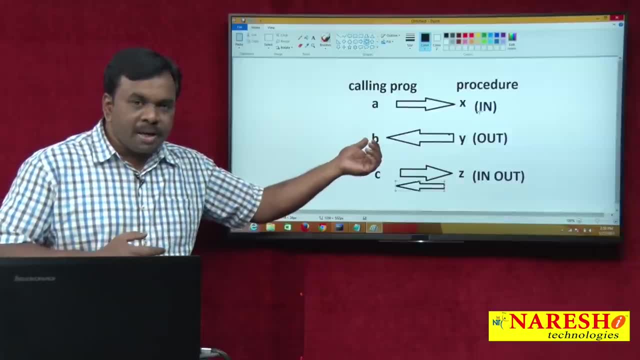 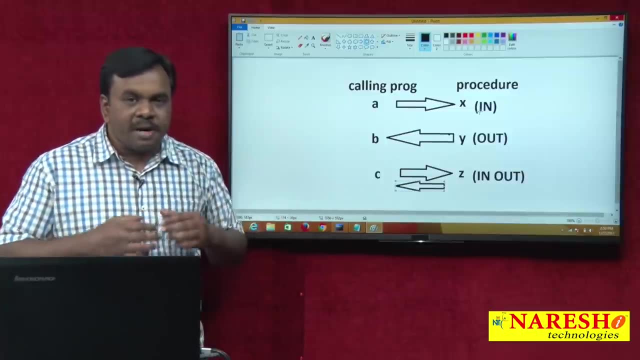 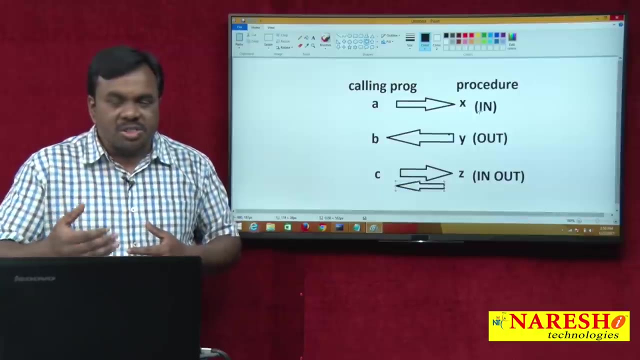 sends value. So the calling program: in the calling program there is a parameter b that receive the value that is coming from y. And next Z is in out parameter. it receives value as well as it sends value. So Z is in out parameter, it receives value as well as it. 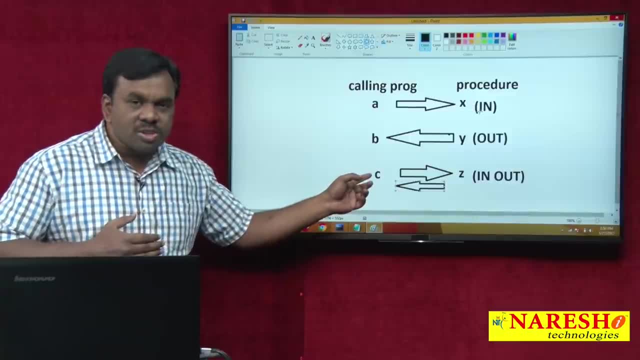 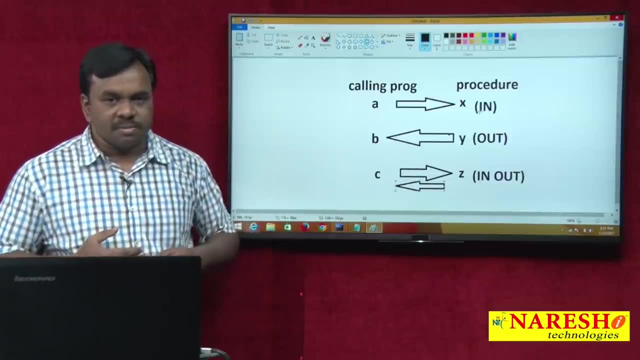 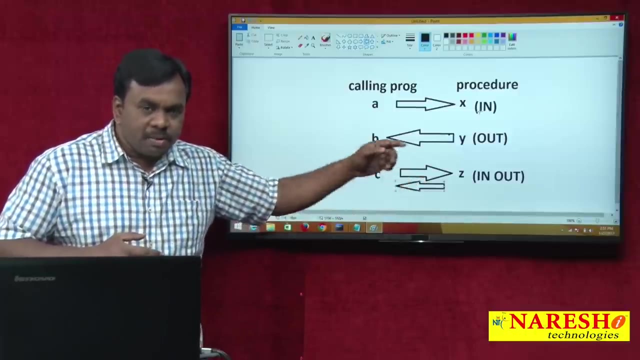 sends value then. So what C receives, first the value of C is sent to Z and the Z value is passed to C, because Z is in, out, it receives as well as sends. So first the value of C is passed to Z and procedure is executed. once execution is completed, the value of Z is passed. 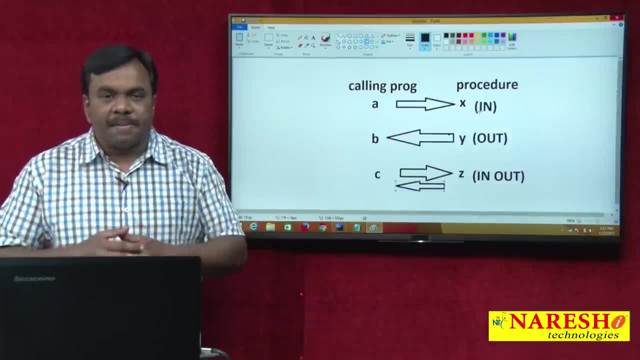 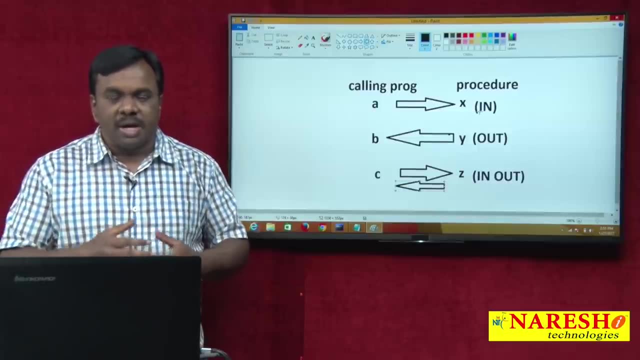 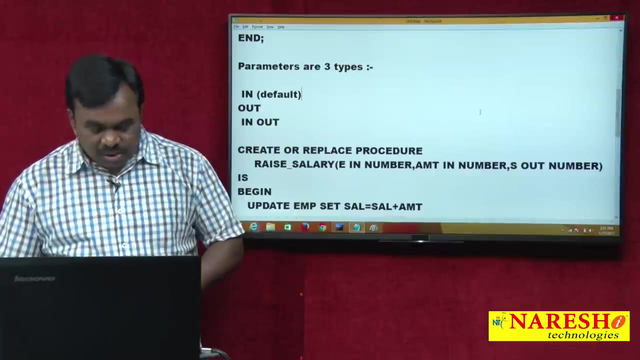 to C. So this is the parameter passing mechanism. So X is in, receives value, Y is out, sends value. and Z is in, out, receives and sends. Now, so let us see one example. So I am creating a procedure, and what for? I am creating a procedure, I am creating a. 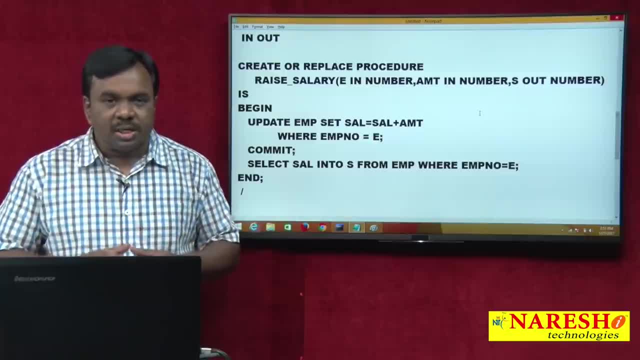 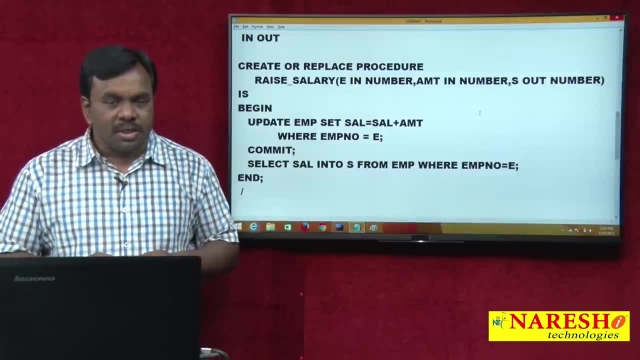 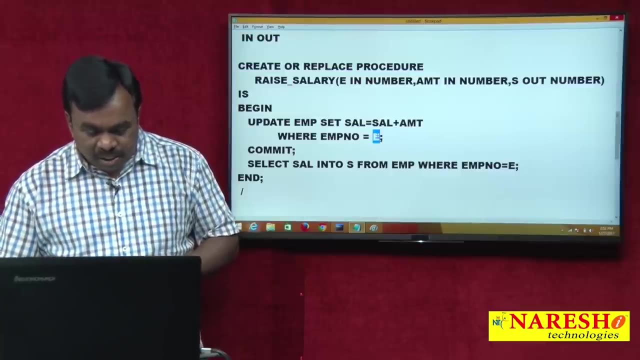 procedure to update the employee salary. This procedure has to increment a particular employee salary by some amount. This procedure has to increment the particular employee salary by some amount, For example here: so the employee number is 7, 8 double 4 and amount is 1000. 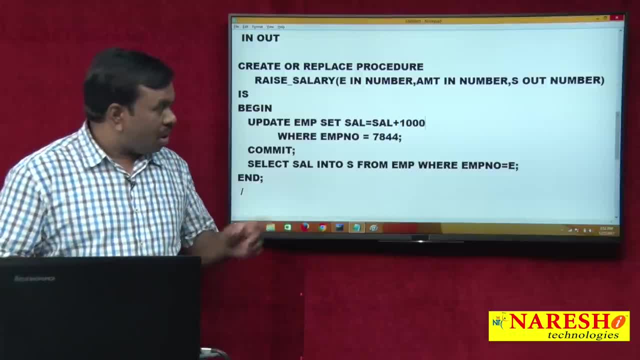 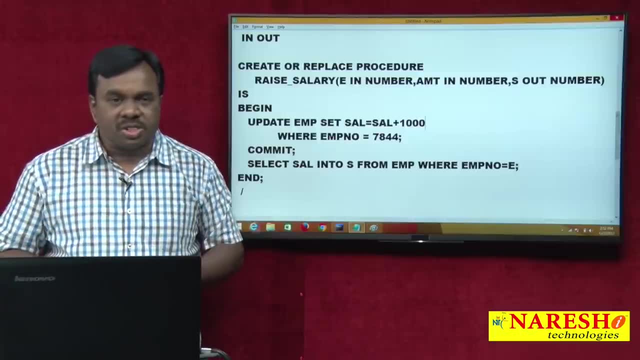 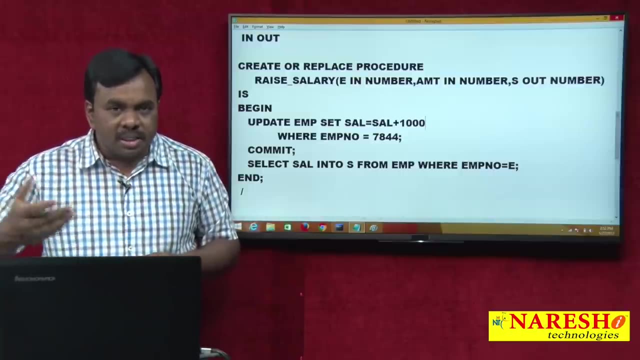 for example. So I am. I am updating like this: update EMP set sal equal to sal plus 1000, where employee number equal to 7- 8 double 4.. So whenever you execute this procedure, this procedure will increment 7- 8 double 4 salary. but so I want to increment a different employee salary. 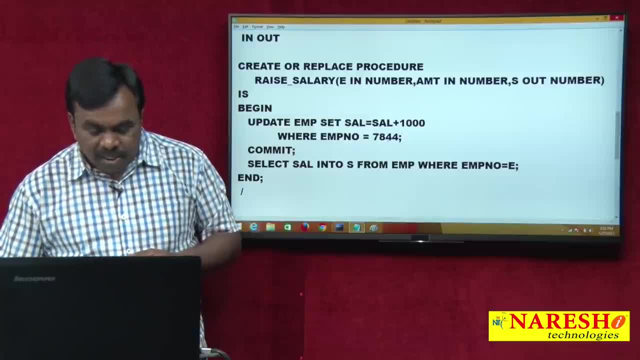 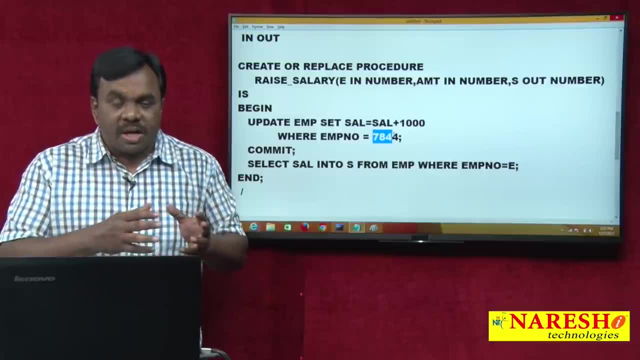 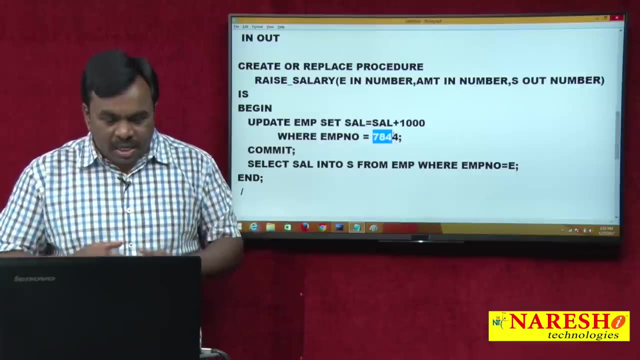 then I do not know this employee number at compile time, I know this employee number at run time. So even this value is passed from A calling program might be Java program, ok, So then I do not know this employee number. I know this employee number at run time. So that is why what I am doing is I am declaring: 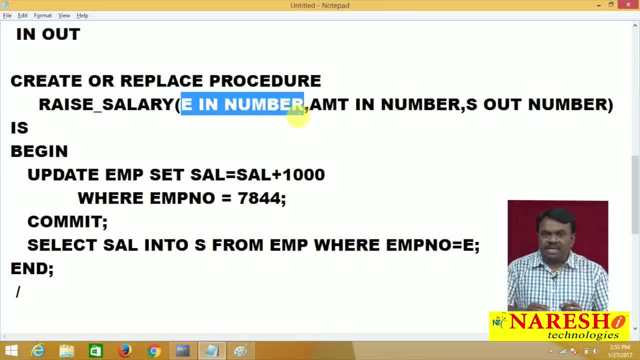 a parameter. I am declaring a parameter that is E. So what is this parameter? type is in in parameter and the data type of this parameter is number. and what did this? E receives this? E receives employee number. where it receives this employee number, it receives employee number from calling program, suppose for? 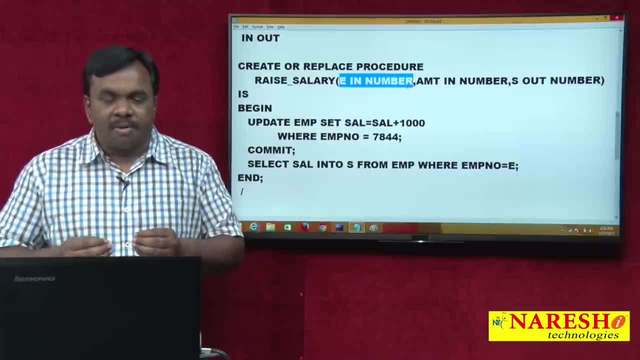 example, the value that he receives is 7, 8, 4, 4, 7, 8, 4, 4 salary should be incremented. the value that he receives 7, 3, 6, 9, 7, 3, 6, 9 salary should be incremented. so, whatever the value, employee. 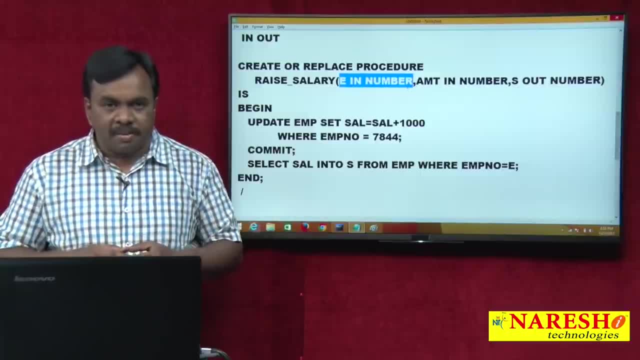 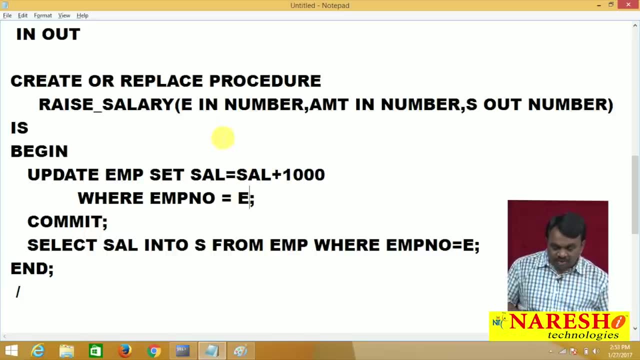 number is positive to e, that particular employee salary should be incremented. so here, in place of this 7, 8, 4, 4, I am using this parameter, e. okay, suppose the value positive to e 7, 3, 6, 9. so 7, 3, 6. 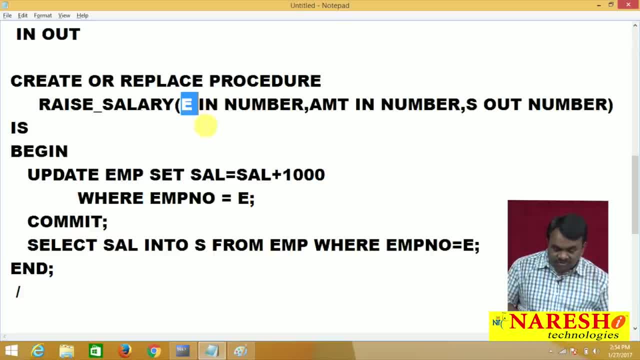 9, salary is incremented. the value positive to e 7, 4, 9, 9, so 7, 4, 9, 9 salary is incremented. so whatever the employee number is positive to e, that particular employee salary is incremented. and one more thing: so this procedure always increment salary by 1000. so but sometimes 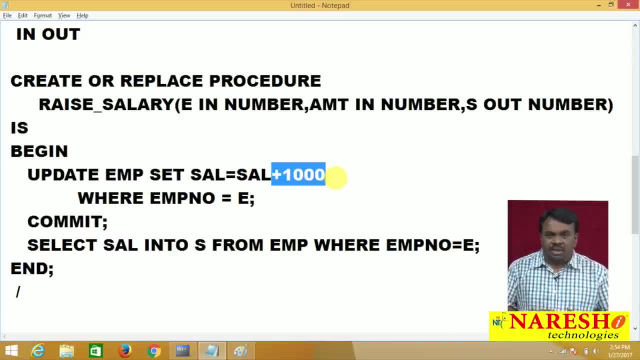 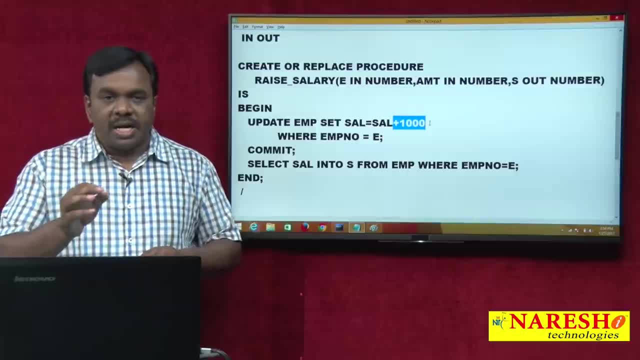 I want to increment salary by 1000, sometimes 2000, sometimes 500, sometimes 3000, but this will always increment salary by 1000. so when you are creating procedures, so what is recommended is try to avoid hard coding better. don't do hard coding, so better to use parameters or variables. so this hard coding 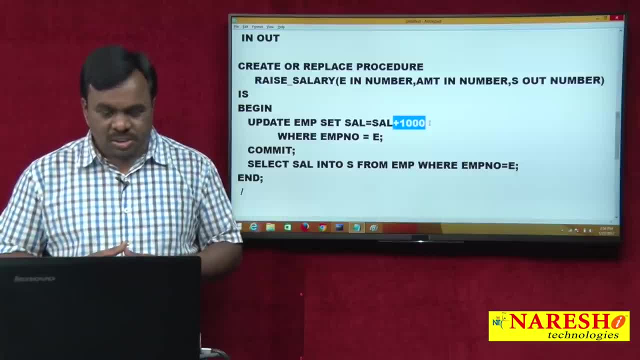 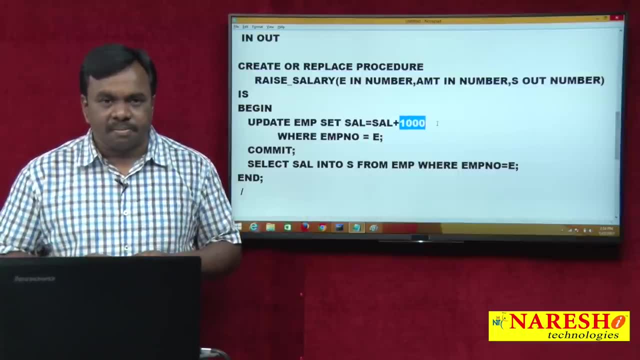 should be avoided better to use either parameters or variables then. so even I don't know this amount at compile time, I know this amount at run time. so at run time this amount is positive. so whatever the amount is positive, that particular that that amount should be incremented. the 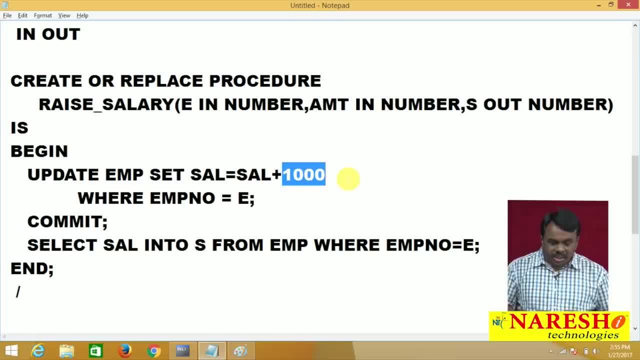 salary should be incremented by that much amount. so then, that's why what I am doing is I am taking another parameter for amount, this also in parameter. this also receive the value. so whatever the amount to this parameter receives, the salary should be incremented by that much value. so here, in place of 1000, I use amt. so using this procedure, you can. 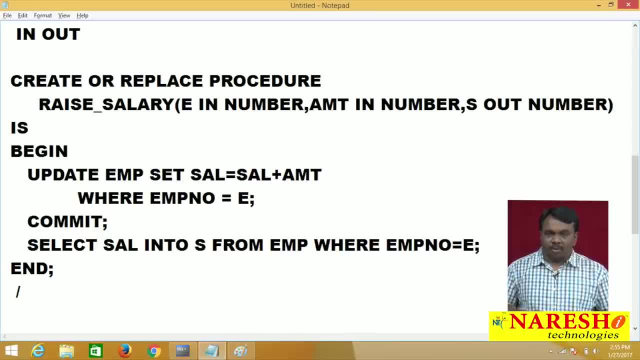 increment a specific employee salary by specific amount. so using this procedure you can increment a specific employee salary by specific amount. so the employee, whatever the employee number, is positive to e that particular employee salary is incremented, and salary is incremented by how much depends on the value positive to this amt. 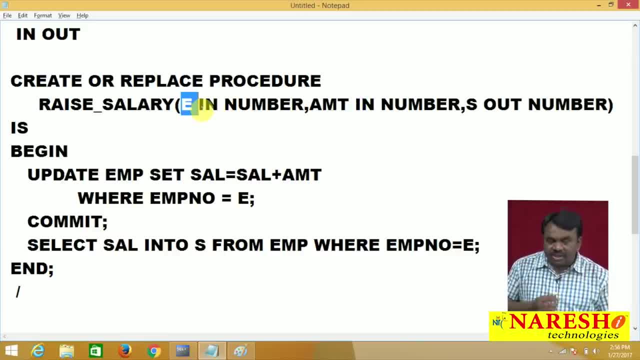 For example, The value positive to e and the value positive to amt is 1000, then 7369. salary is incremented by 1000. the value positive to e is 7499 and the value positive amt is 500, then 7499 salary. 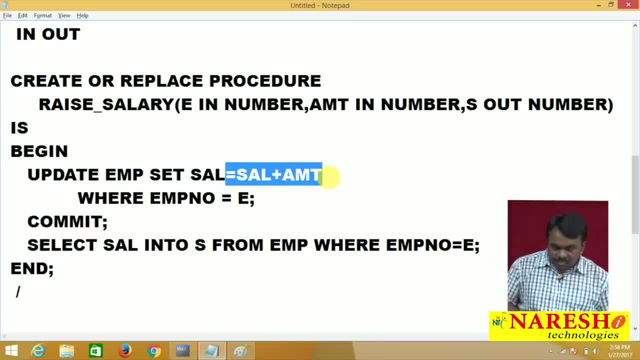 is incremented by 500. okay then. So I am incrementing the salary one. this update is completed. then I am executing this commit after update. Amt the commit. So then this update becomes what? permanent. So this update is saved. 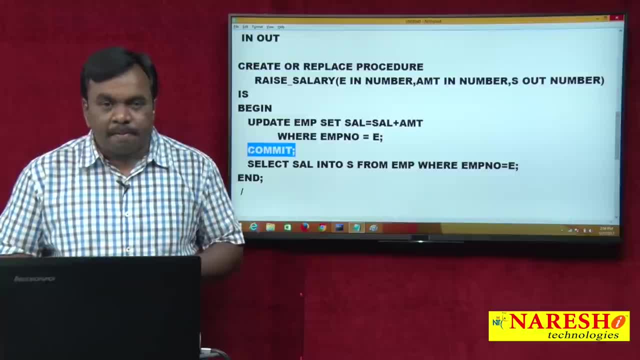 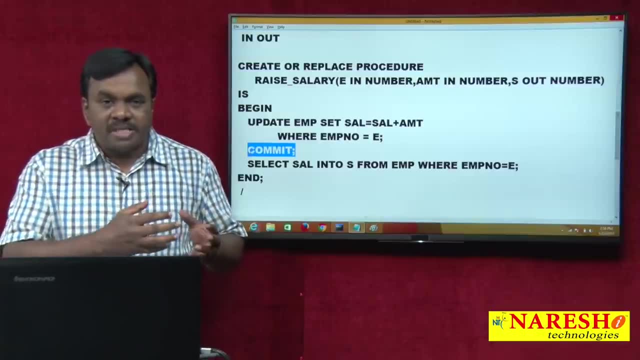 After updating the salary is modified, the employee salary is modified. I want to send this new salary to the calling program. So the calling program is expecting the modified salary, the new salary of the employee. Updated the salary and after that, the operation is committed. 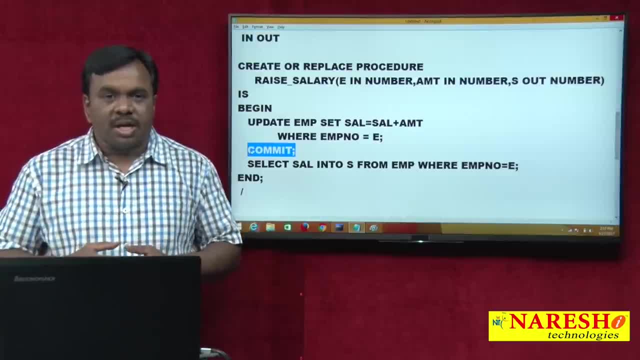 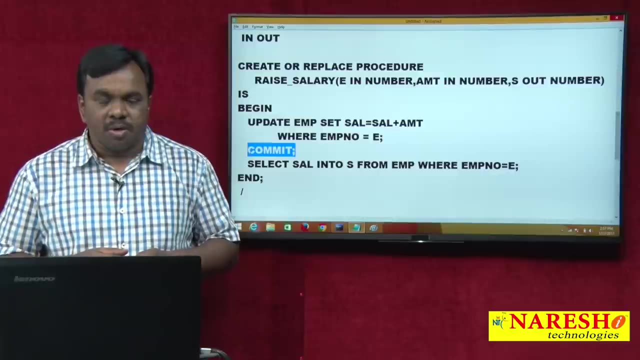 then next I want to send this new salary to the calling program. So what calling program is expecting is calling program is expecting new salary, that. So if you want to send something from procedure, then take out parameter. You want to receive something coming from calling program. 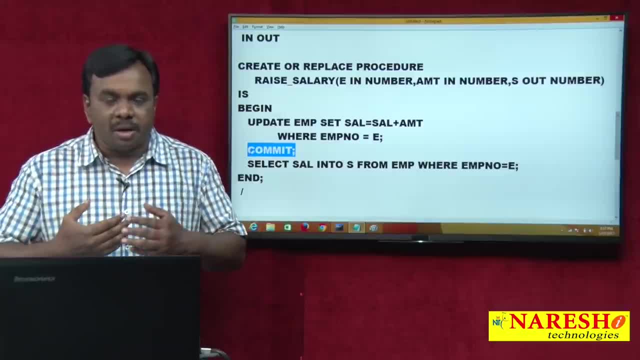 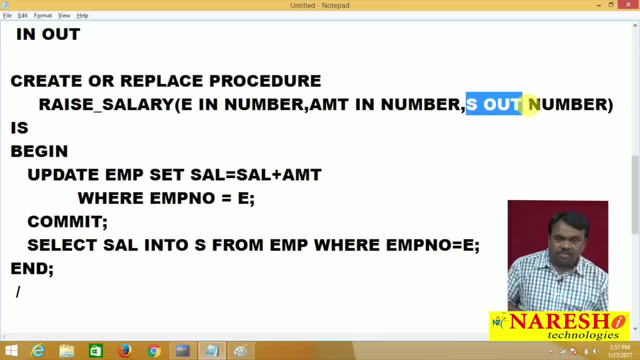 take in parameter. If you want to send something from calling from procedure, take out parameter. So here I have taken one out parameter. The out parameter is the out parameter. So the out parameter is the out parameter. So what for you have taken this out parameter Because so I want to send the updated salary. 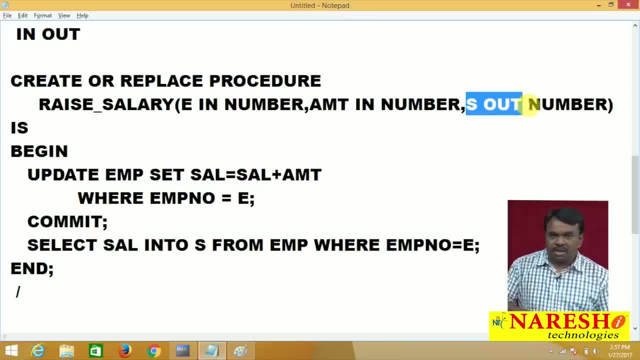 to the calling program. So I take an out parameter, Take out parameter. whatever the value you want to send, assign that value to the out parameter and the whatever the value is assigned to out parameter, that value is automatically sent to the calling program In the calling program. 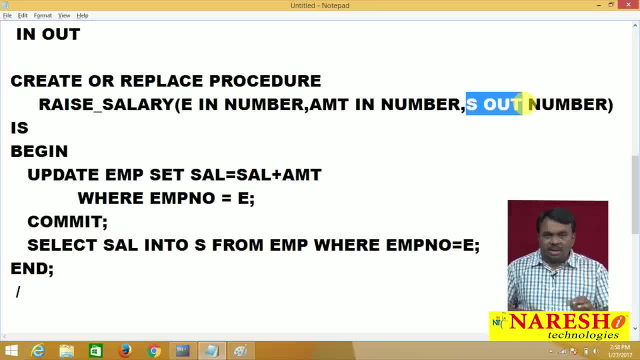 you can receive that value. So your duty is: declare an out parameter, assign the value to the to the out parameter. whatever is assigned to the out parameter, that file is automatically sent to the calling program. So next what I am doing is I am getting the updated salary. 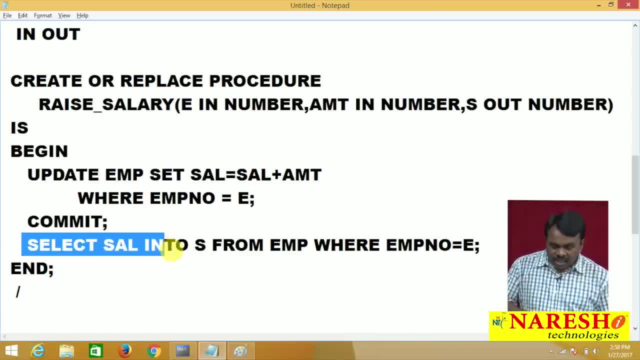 So, using the select statement, I am getting the updated salary. and updated salary is assigned to S. what is this? S is S is out parameter, So getting the new salary. the new salary is assigned to the out parameter whose employee number equals to E. that So the updated salary. 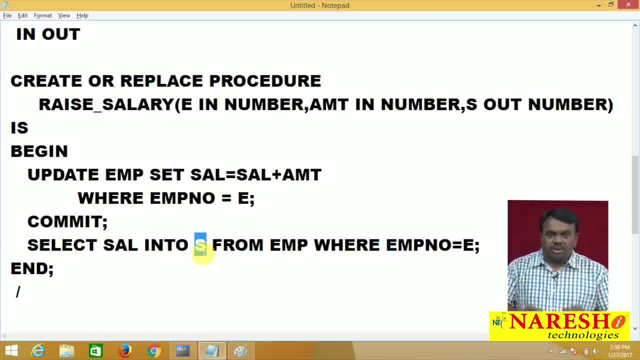 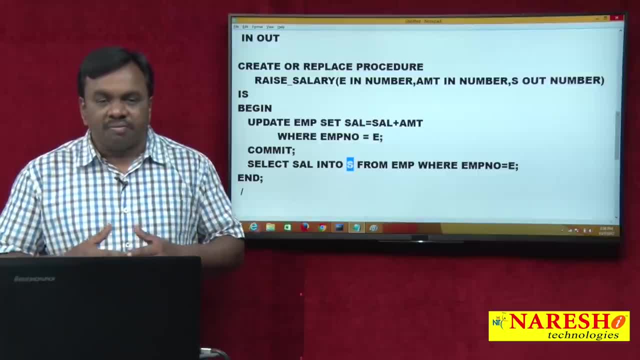 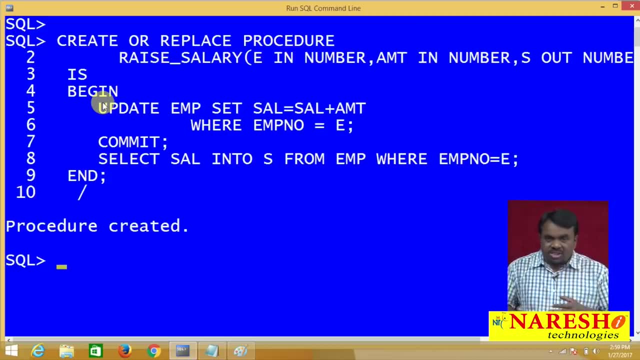 is selected and the updated salary is assigned to. So this out parameter S. So let us create this procedure first. we will create this procedure after creating this procedure and we will execute this procedure. So I am going to SQL plus. So procedure is created. procedure is created, means. 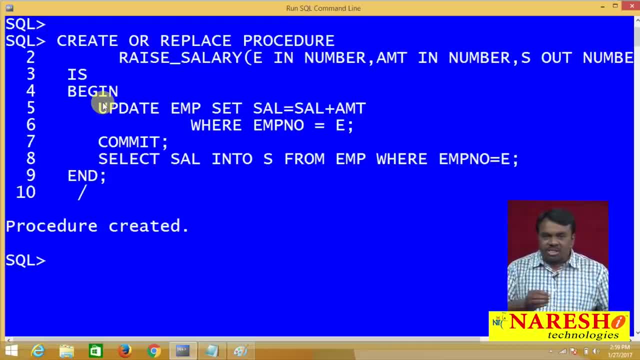 this particular code. whatever the code you have written, that code is compiled and this is stored in database. Now, whenever you want, you can execute this procedure. So, whenever you want, you can execute this procedure. then now I want to execute this procedure. So to execute this procedure, So you can execute this procedure from SQL prompt, or you. 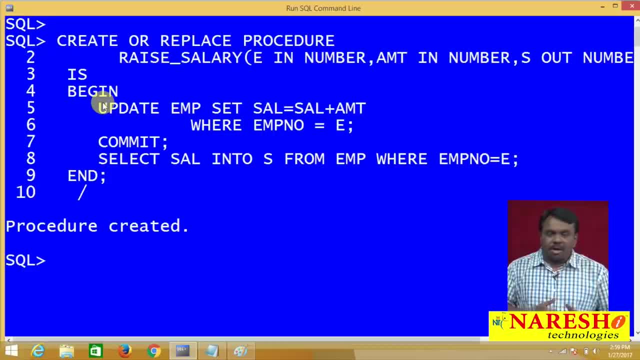 can execute this procedure from another PL SQL program, or you can execute this procedure from any front end application. You can execute this procedure from SQL prompt, or you can execute this procedure from another PL SQL program, or you can execute this procedure from any front end application. 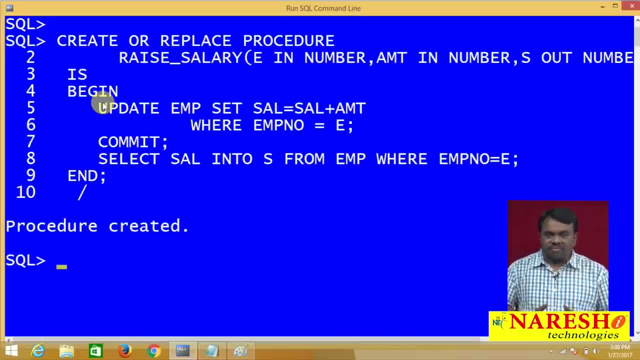 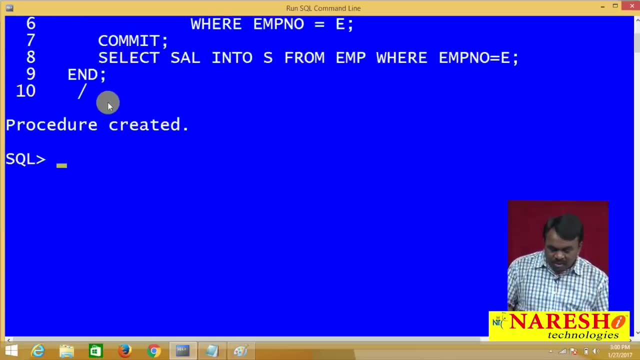 So suppose let us see how to execute this procedure from SQL prompt, because in procedure is created with out parameter, So out parameter send the value. here I have to receive the value. to receive the value, I declare a variable. So I am declaring a variable, how to? 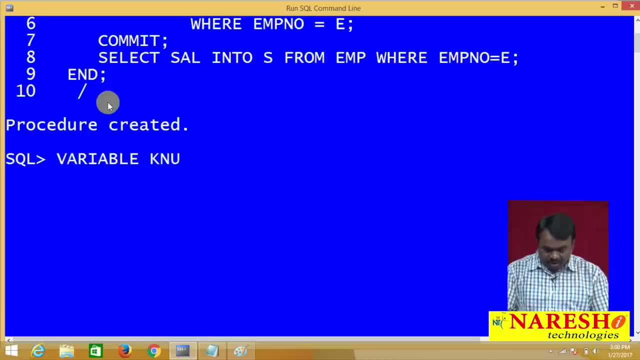 declare variable SQL prompt variable k number. So I am declaring this variable to receive the value that is coming from procedure, because procedure is created with out parameter that send the value. to receive that value, I am declaring a variable k, then Next execute procedure. execute. so what did I command? To execute the procedure, execute procedure. 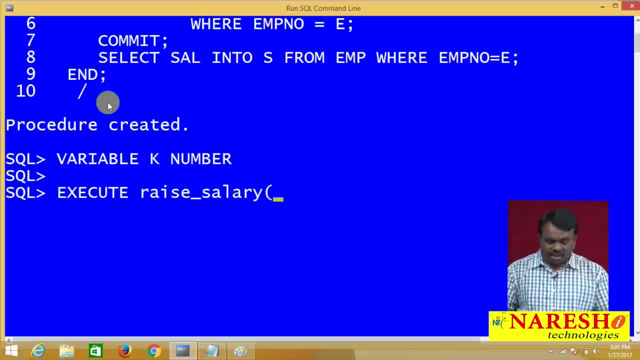 name. what is the procedure? name is price salary, then. so pass employee number. and one more thing before executing the procedure. let us see what is the salary of the employee, So select employee number. salary from EMP. so what is the salary of 7369? the salary of 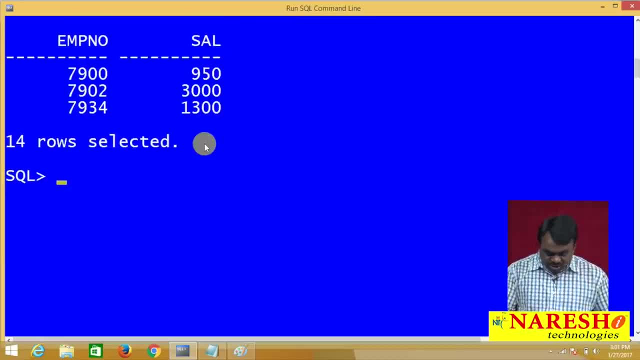 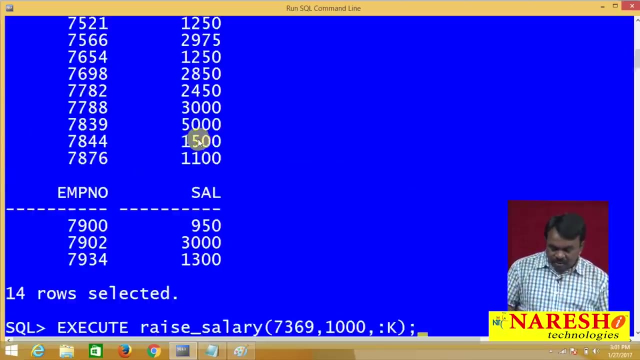 7369 is 800. let us execute the procedure. execute procedure: name is price salary, So employee number is 7369. suppose 1000. next colon k: I declare a variable, the variable is k and what this variable is called bind variable and the bind variables are accessed. 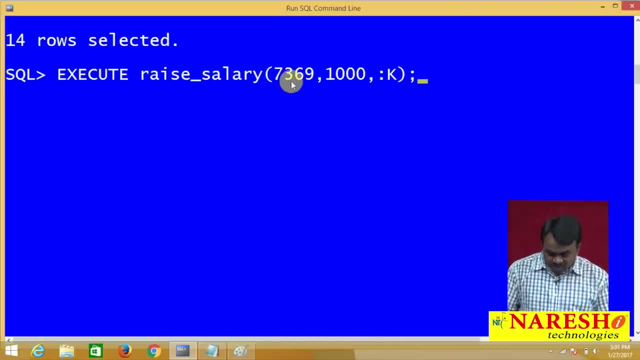 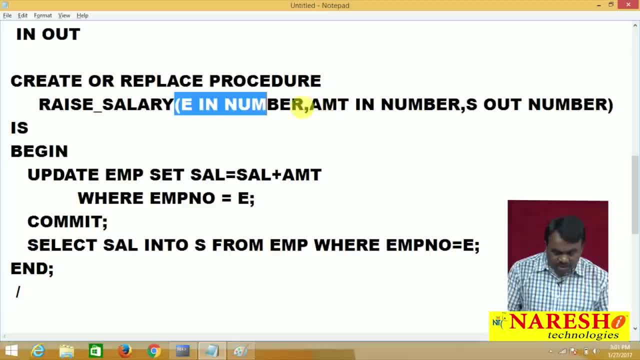 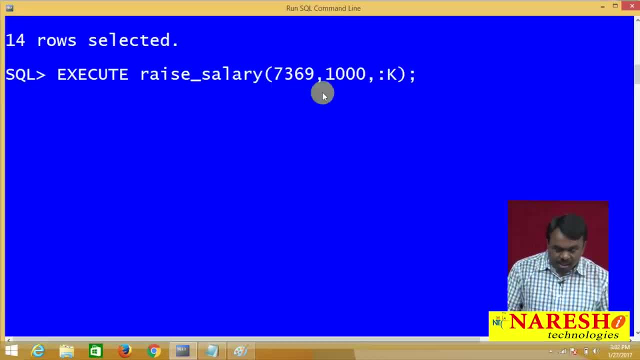 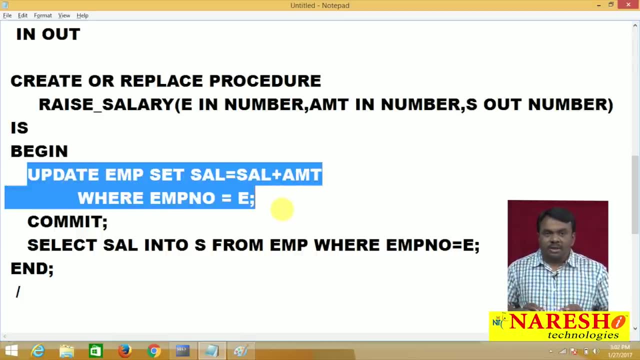 This 7369 is positive to E and this 1000 is positive to AMT. So first, this value 7369 is positive to E and this value 1000 is positive to AMT, and procedure is executed. So what this update command is doing? this update command is incrementing 7369 salary. 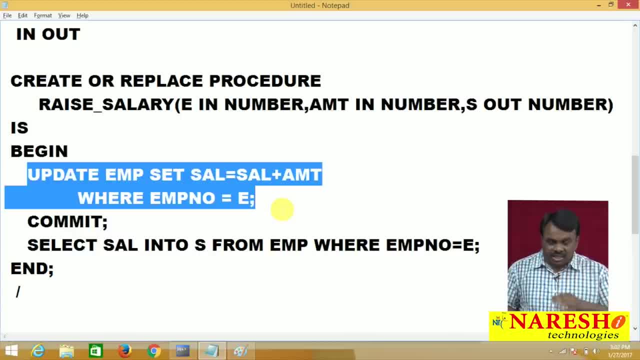 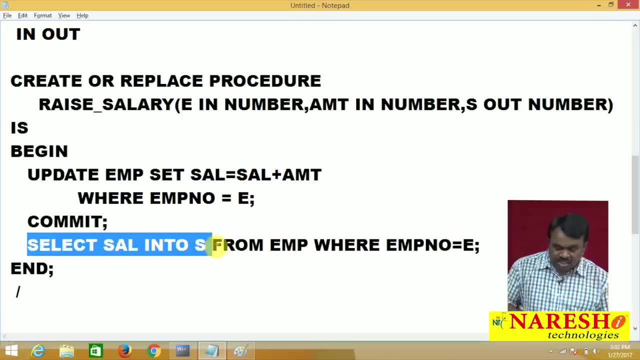 by 1000.. So 7369 salary is incremented by 1000.. So so here, E is replaced with 7369.. KMT is replaced with 1000.. So 7369 salary is incremented by 1000 and the operation is saved. and what this select statement? 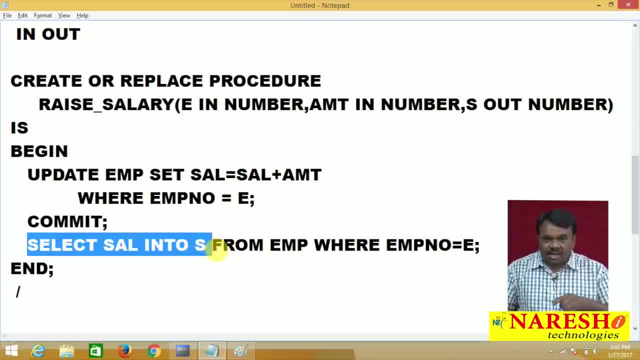 is getting the new salary, the actual salary of the employees, 800 plus 1000.. So incremented by 1000. now it is updated with 1800 and the select statement is selecting the new salary. that is 1800 and that value is assigned to S. what is this? S is, S is out. 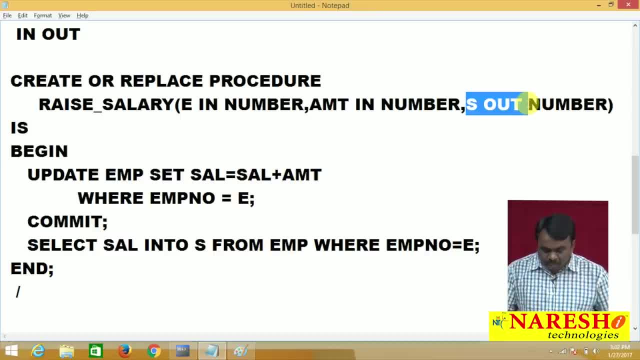 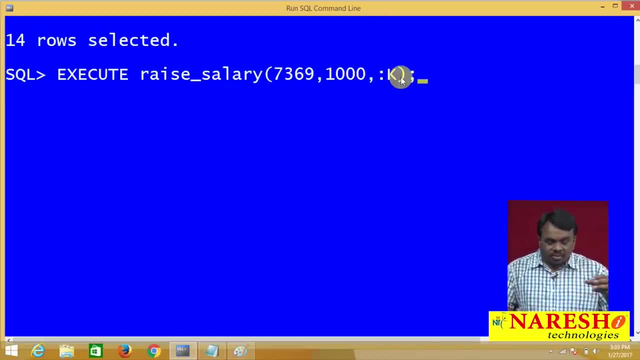 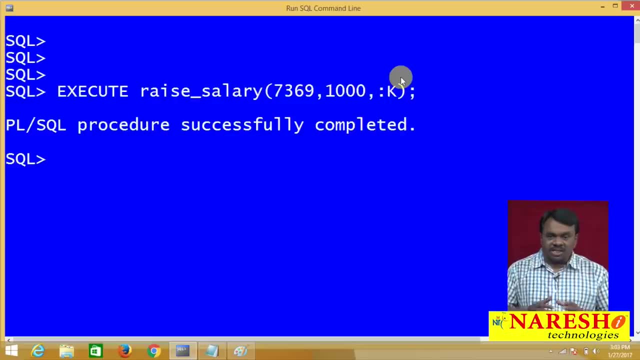 parameter and this out: parameter: value sent to, So in the calling program, in the calling program K will receive that value. So procedure is sending the value So that value K will receive that value. So execute the procedure and I am executing the procedure. PLS skill project successfully. 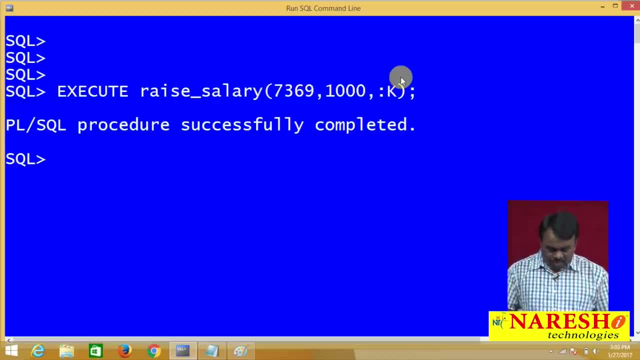 completed. Just go and see the 7369 salary and select EMP- NO sal from EMP. select EMP: NO salary from EMP. So otherwise You can. It is. it is updated in the table. otherwise you can also see the new salary. the new salary is passed to K. if you want to print the value of K, print to colon K. 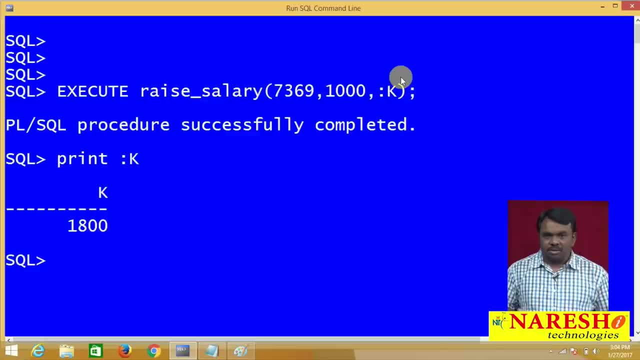 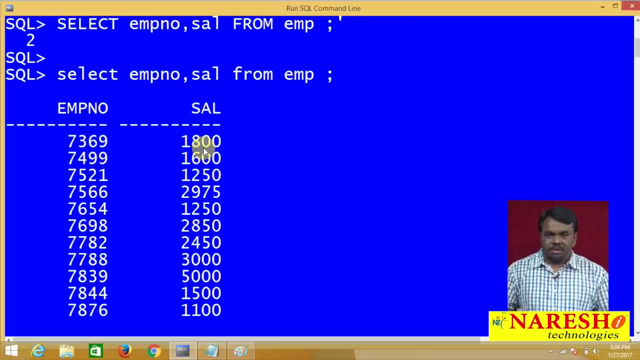 So what? the new salaries? 1800.. So it is. it is procedure is sending the updated salary so that K will receive that value and printing the value of K and even if you go and see the salary in table from EMP, So 7369 salary is updated with 1800.. 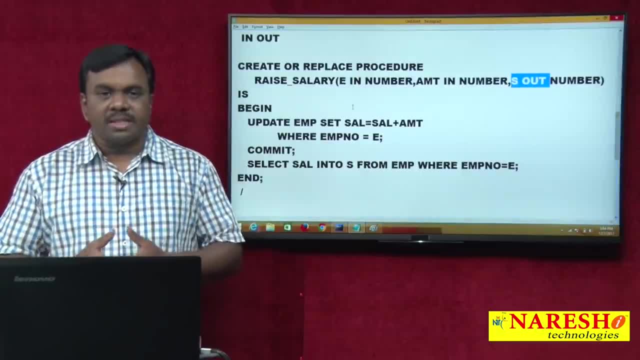 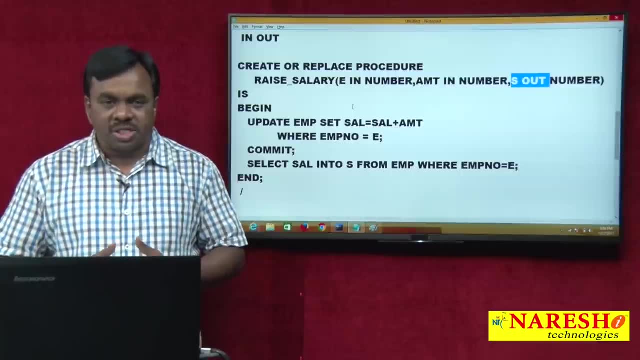 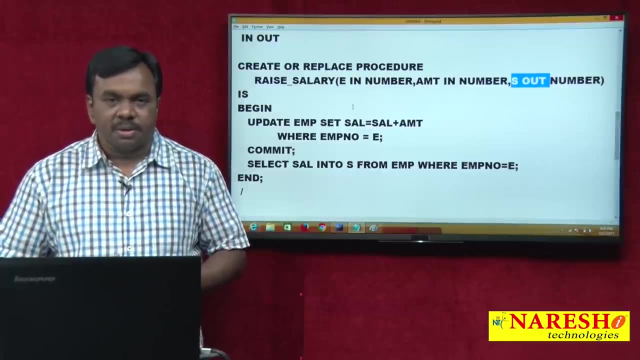 So this is like how to create a procedure and how to execute the procedure in today's this video. So you learnt how to create a procedure and how to execute the procedure, that is, how to use in parameters, out parameters and in out parameters. So thank you for watching this video. for more videos, subscribe to Naresh IT. 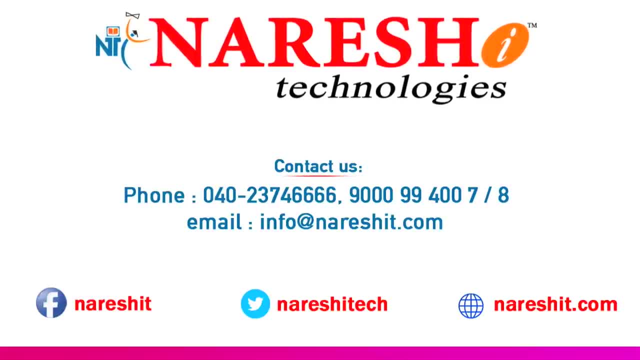 Thank you for watching this video.